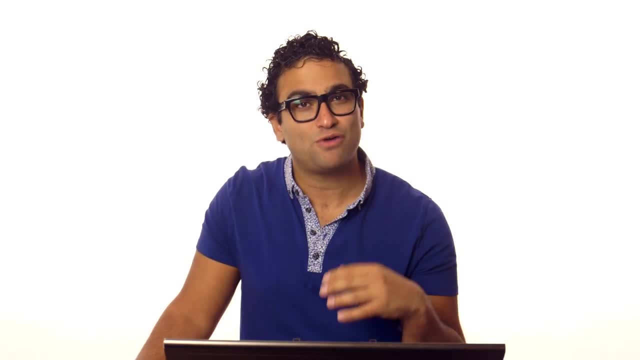 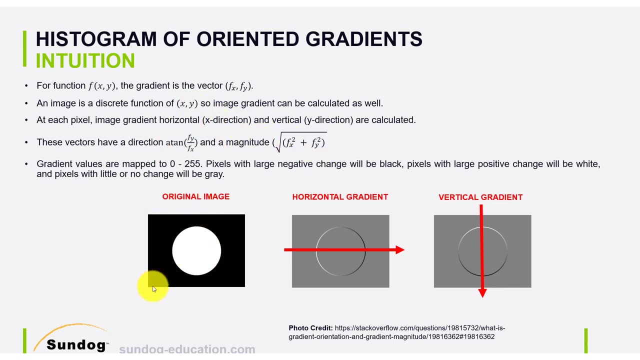 want to jump directly into HOG features, because here I'm just going to cover the basics of how to. what do you mean by gradient within an image? okay, Let's take a look at a very simple example. Let's assume that I have my original image, which is kind of, you know, all black and it has kind of a 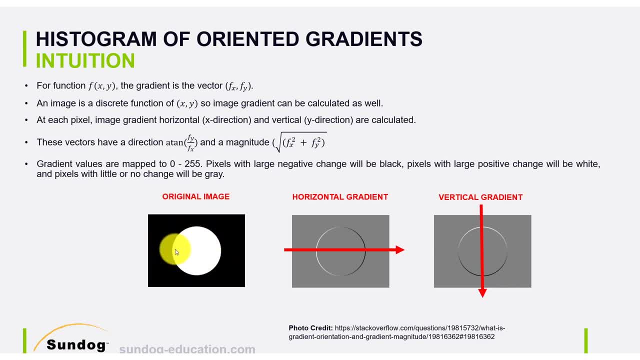 white circle in between, in the center. okay, and what I want? that I want to calculate the gradient in the x direction. Okay, what's called horizontal gradient gradient, okay, Okay, so what we're going to do here? we're just going to go walk from the left to the right, scan it here. all of it is black, right, so we're. 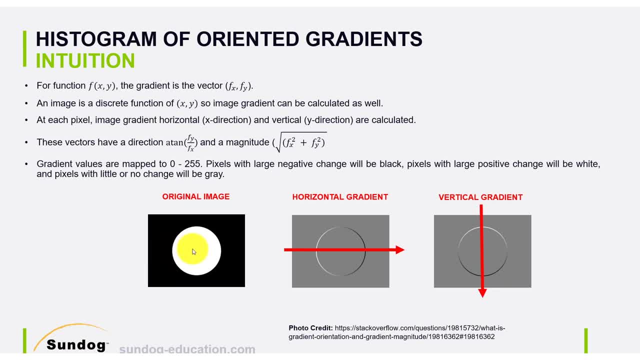 going to go zero, zero, zero. all the pixels are zero. and then suddenly I'm going to see white pixels, which indicates 255 or white color or a bright color, So I'm going from zero. suddenly I saw one. so that means I'm going from zero. and suddenly I went to one, which means there's a big 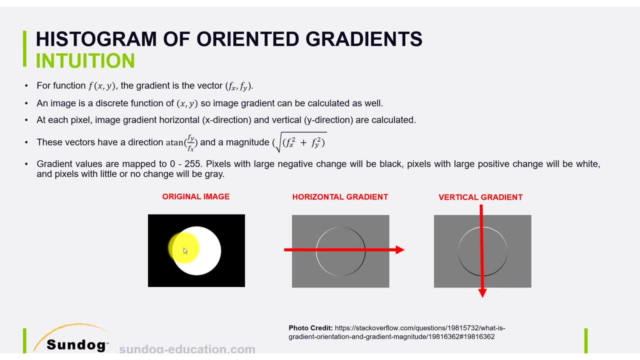 difference in magnitude, going from very small value to a very large value, right? So that means I can find there is a positive gradient and that's simply indicated here in that gradient image by white color here indicating there is a positive gradient, okay, indicating, okay, this in this specific 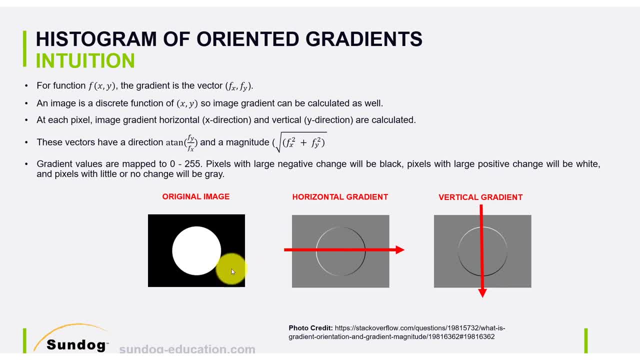 point there is a change in the intensity in the original image. Okay, let's keep going. all right. as you move forward here you will see it going from one to the other. So I'm going to go to the left and then I'm going from white. suddenly you hit black color. so you're going from 255 suddenly. 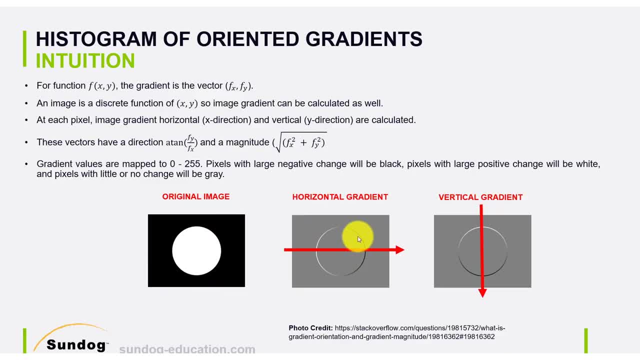 you had to go to zero color, okay, and that's why that's been indicated by kind of a negative gradient. you're going negative, going down, and that's why here you will see this thing get indicated by a black color, indicating kind of a negative pixels or negative gradient. okay, all right. 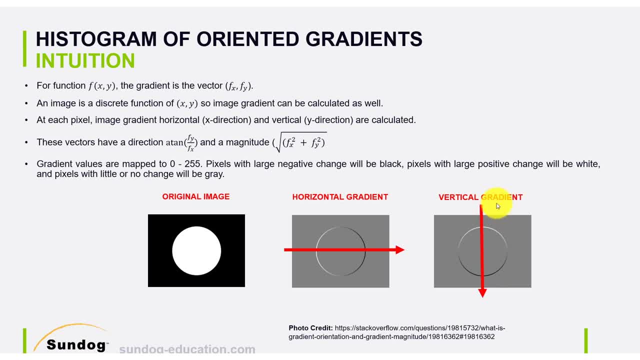 very interesting. let's do the exact same stuff, but for a vertical gradient. so you're going from up down. so again you guys can see, here you're going to see there is white because you're going from black to white To black. you can see there's a negative gradient or kind of a black values here indicating negative. 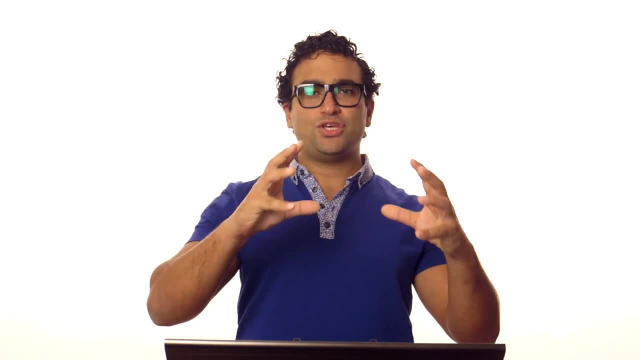 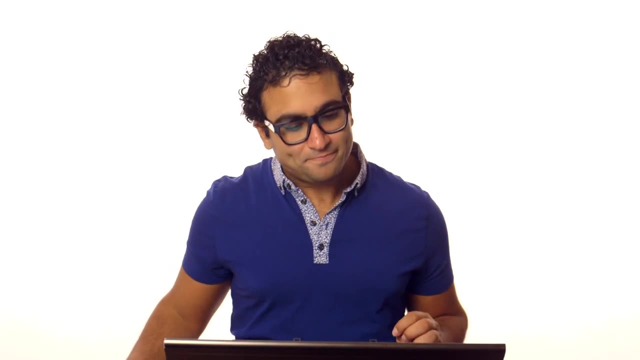 gradient and that's how you can- you kind of you take an original image- you can create your horizontal gradient and your vertical gradient. that's the first basic foundations of Hawk features. okay, all right, so that's first step. okay, what I'm going to do with this, like what's the 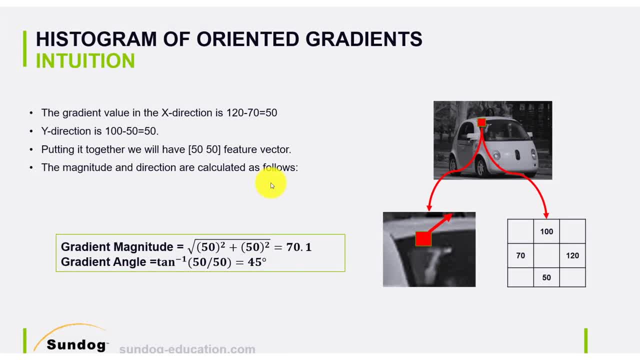 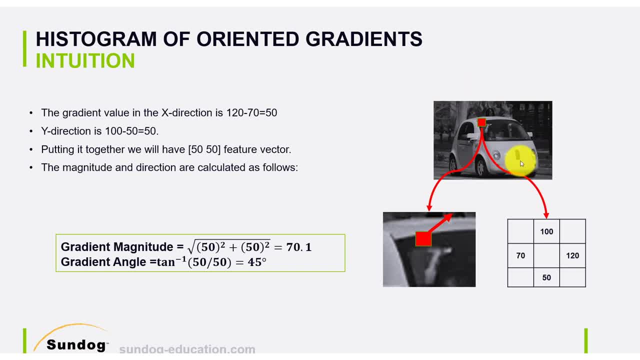 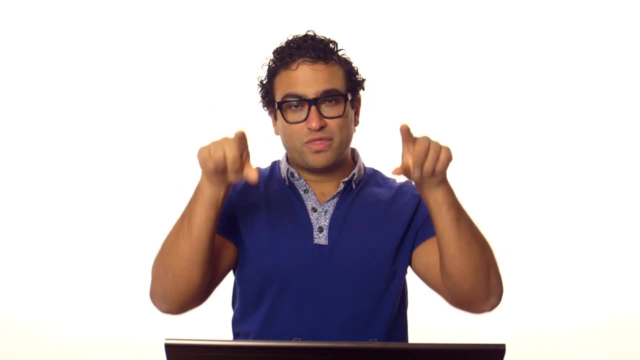 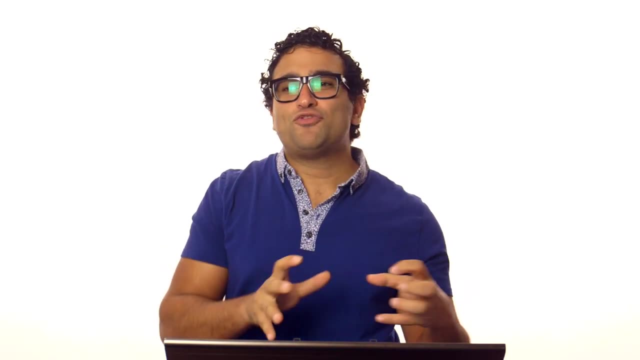 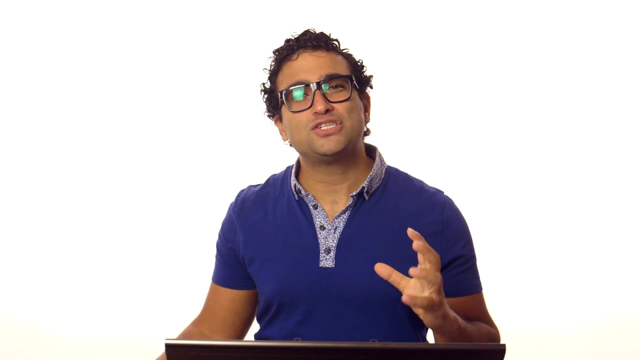 you know like kind of these couple of cells, a couple of pixels within an image, in a different representation, in a very compact representation in which I can feed, for example, to a machine learning algorithm that can learns easily and fast, very, in a very efficient way. Okay, And that's the beauty of histogram-oriented gradient. It's kind of you know you're applying. 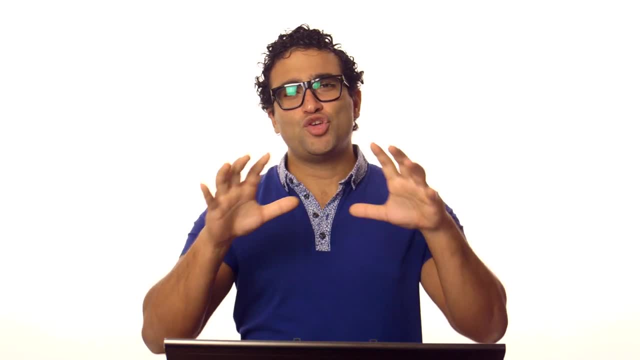 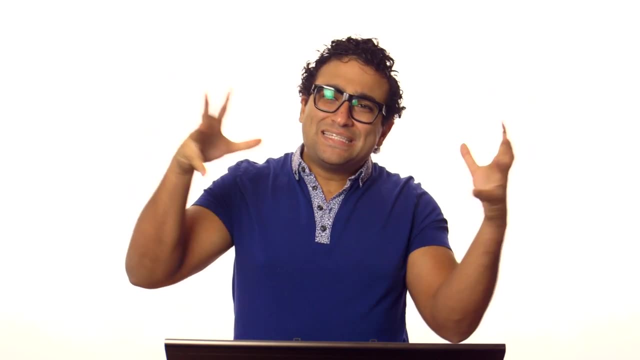 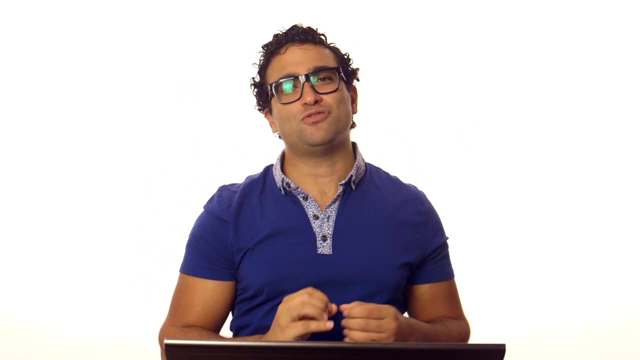 like you are zipping a file in a way. You're getting your file, You are zipping it, You're just removing all the unnecessary information. okay, Condensing down a lot of information from, let's say, 64 by 64. You're condensing it down to, let's say, nine values in a way. 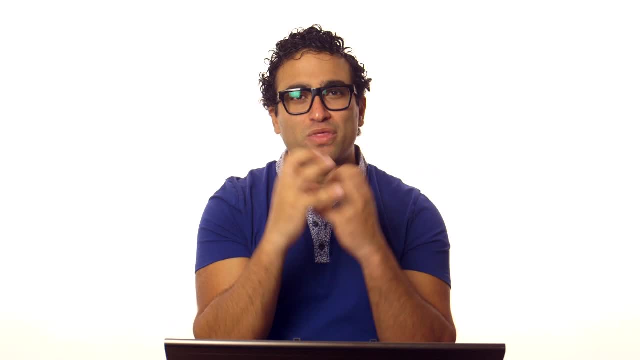 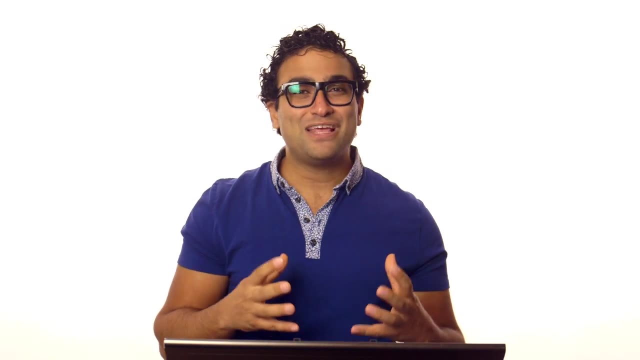 okay, And that nine values just represents all the features within the image. It's really powerful And I'm like really kind of more. yeah, I think you guys can feel it. Just I'm a little bit passionate about that topic. It's very interesting and it can show you after how can we actually 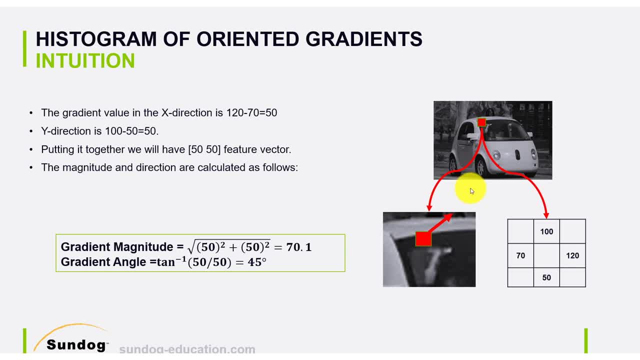 train a machine learning classifier to detect objects using the histogram-oriented gradients. okay, So let's assume that I zoomed in within that pixel, as you guys can see here, and that's pretty much my pixel. okay, That's kind of my zone, That's my area. So the pixel under 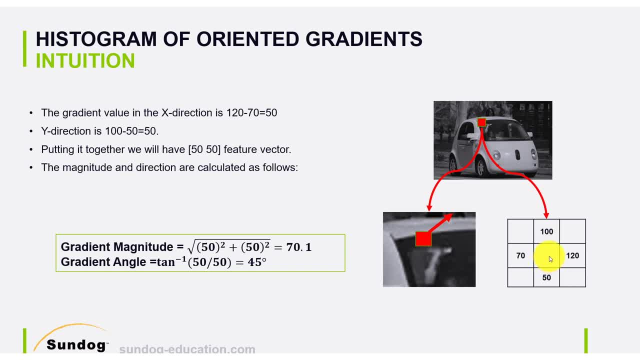 consideration is this pixel, and I'm looking at the pixels around it per se. So here I have 100,, 120,, 50, and 70. So how can I calculate the gradient in the x direction? What I could do is I could simply subtract. I'm moving this way, So I'm going to subtract 120 minus 70,. 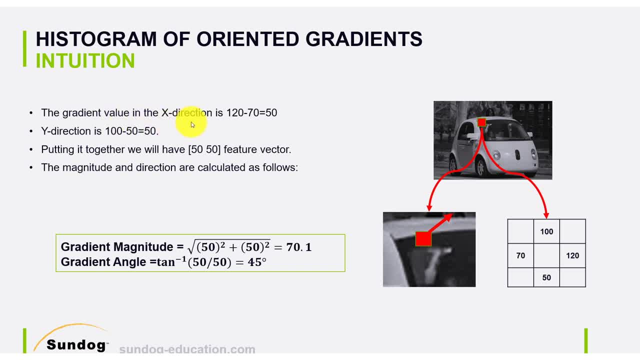 right, And that will be the gradient value within the x direction. so 120 minus 70, which is equal 50, okay, All right. Okay. The next step is I'm going to check the gradient in the y direction. I'm going from 100, okay, Again. 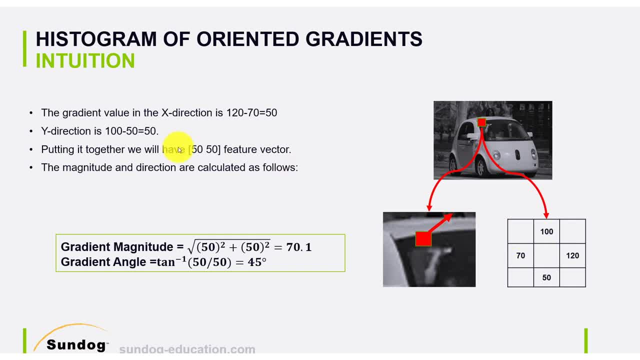 I'm going to 50, let's say to 100.. So I'm going to go, okay, 100 minus 50. That will give me again 50,. all right, Let's put it all together. Then I have pretty much kind of a vector that. 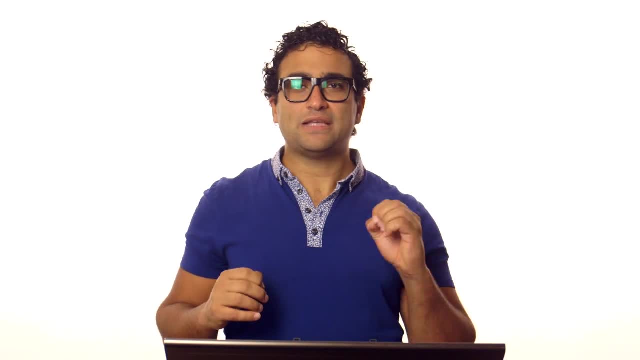 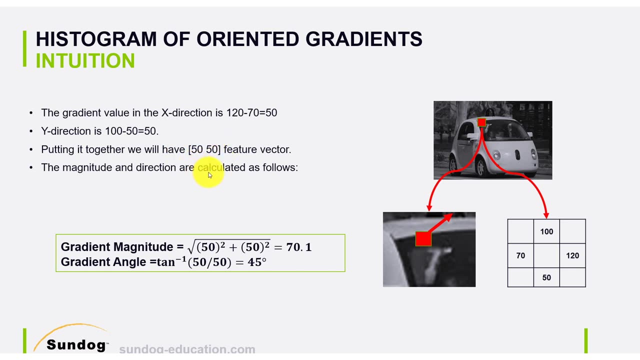 tells me: okay, that's my gradient in the x direction and in the y direction. So now I have a gradient 50 in the x and 50 in the y. all right, Once I have these two pieces of information, actually, I can just a little bit go back to the other mathematics that I discussed before. 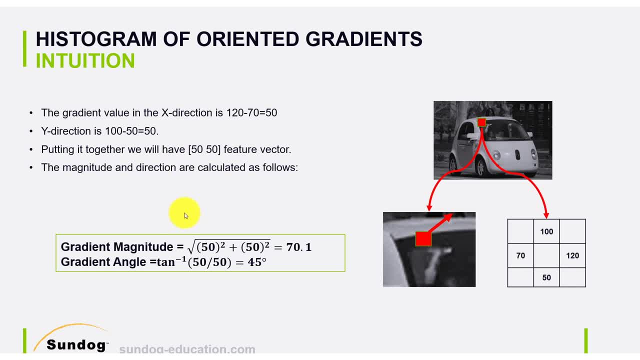 I can get the overall gradient value or gradient magnitude and gradient angle, if you guys recall before. So I can get the square root of 50 square plus 50 square or kind of gradient x square plus gradient y square under the square root will give me 70.. 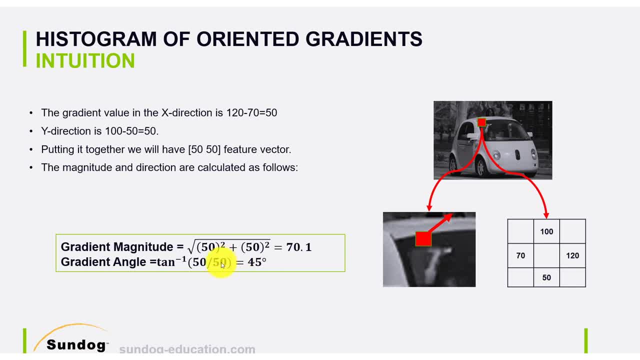 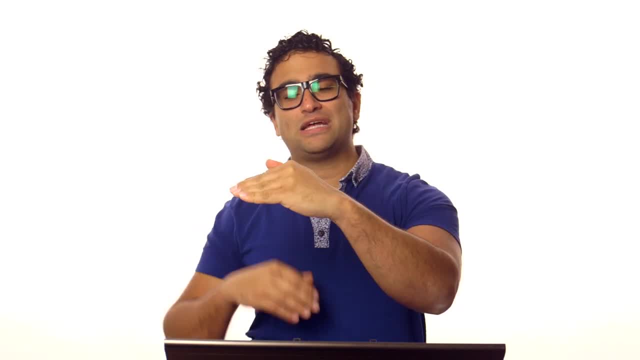 And then I can get the gradient angle too, which is, you know, indicating there is a 45 degrees, And that's the beauty of it. Now we can represent, instead of having gradient separately in the x direction, gradient separately in formation, the y direction. I mix them together and I got. 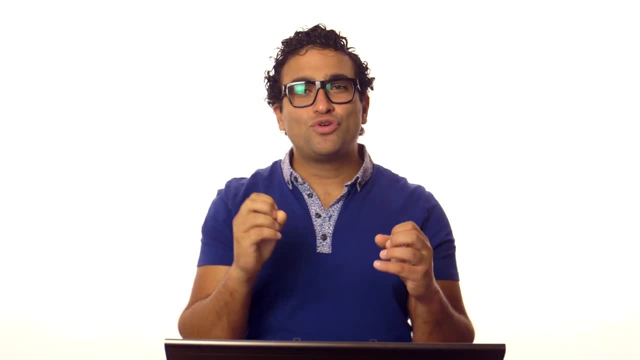 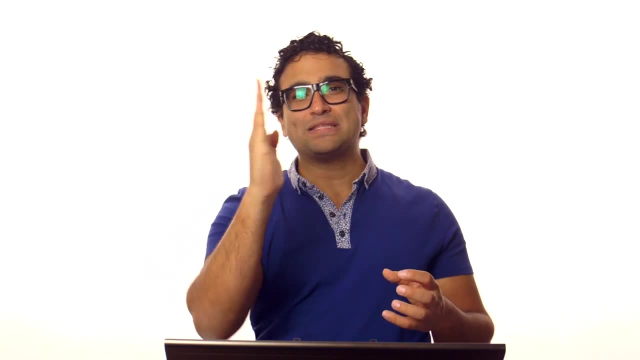 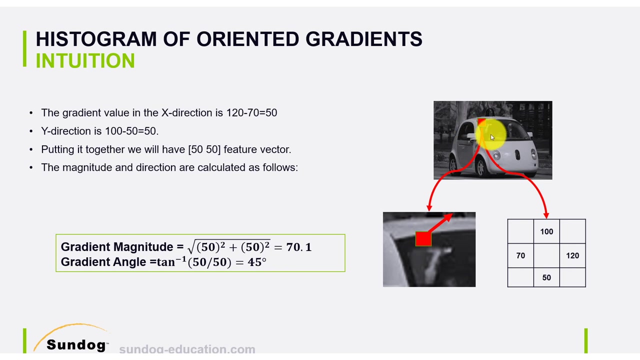 a kind of a vector, And that's where the histogram of kind of oriented gradients- oriented gradients- you're looking at gradients in a kind of orientation- What angle are you looking for? Okay, So here, simply put, I can represent these couple of pixels in a way, in a kind of 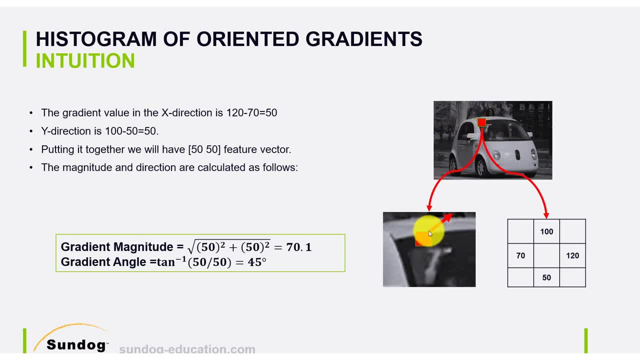 you know, like a magnitude indicating the length of my arrow. If that arrow is long, that means there's a higher magnitude value. If it's a little bit short, that means maybe like 20 or maybe 10, and then I can indicate direction too. Now I have 45 degrees, which indicating I have 45 degrees. 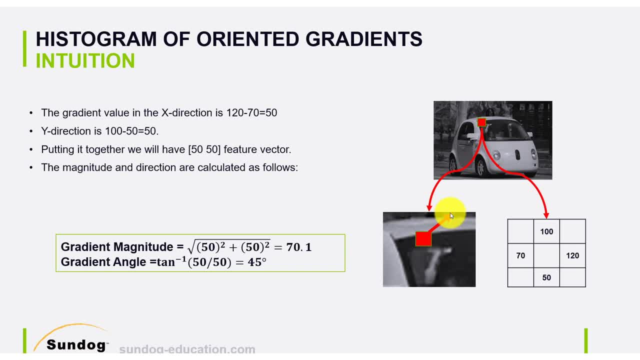 which is perfect. That's amazing. All right, Again, I didn't get like what I'm going to do with this. Okay, Moving forward. First, that's how I obtain the oriented gradient parts. Now I have gradients that has been oriented with different angles. Let's get the histogram of it And that's. 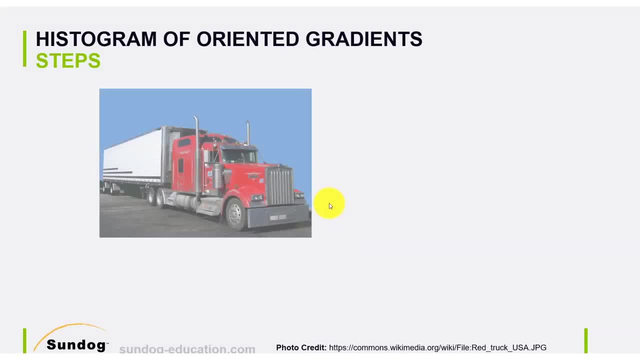 again. you know another fascinating idea. So how can we do this? Let's assume again, let's take a look at it practically. For example, let's assume I have my truck, First step if I'm going to use. let's say I have to. 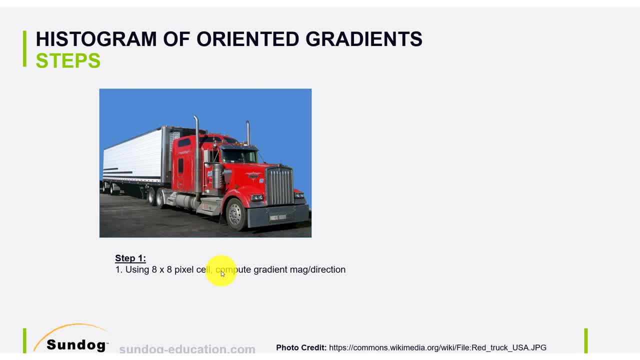 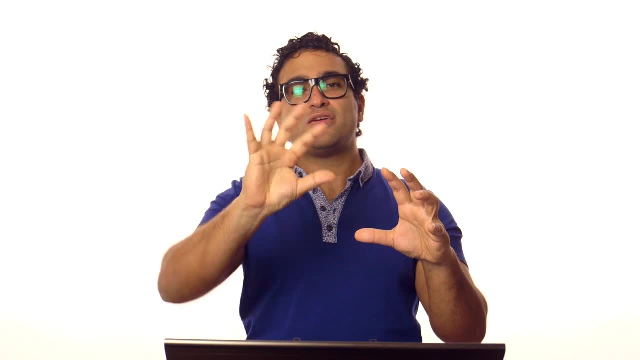 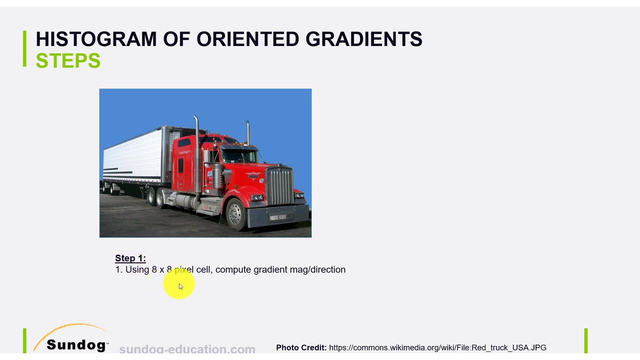 define my histogram of oriented gradient, I have to identify kind of a zone or a cell. we'll call it cell area. In this area I'm going to be representing it by kind of the by a hog, by a hog feature, or histogram of oriented gradient feature. Okay, So, using 8x8 pixel, I'm going to 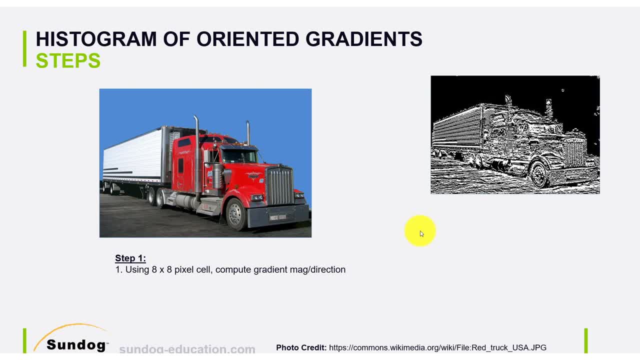 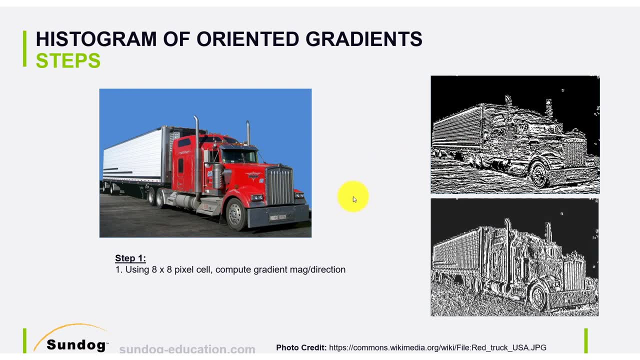 compute gradient and magnitude direction. All right, So, simply put, I can take the image I'm going to get. I'm going to get this one. That's gradient x, That's sobel x. Okay, I'm going to get sobel y. If you guys can see the derivative, it's kind of, you know, like vertical. So that's sobel y. 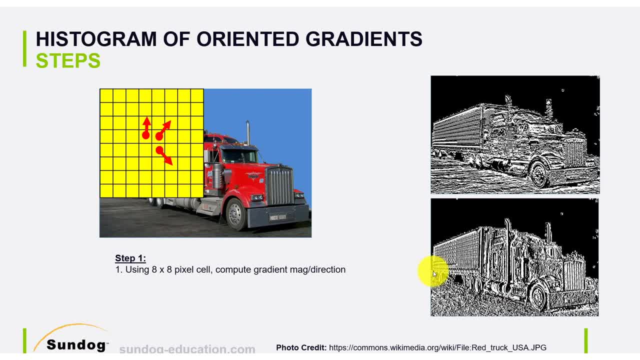 or gradient in direction y, And then afterwards what I'm going to do is I'm going to take, mix them together. I'm going to get the gradient in the x direction, gradient in the y direction, So for each pixel now I have gradient in the x, gradient in the y. All right, perfect. Next step. 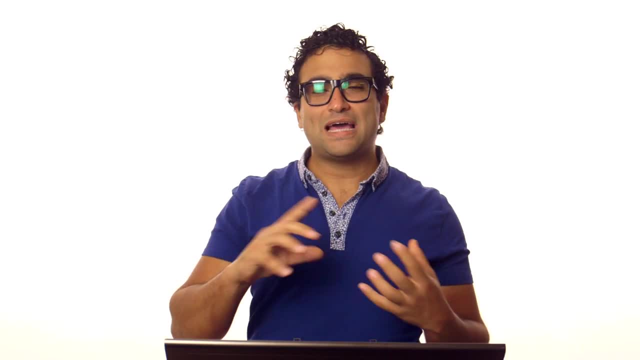 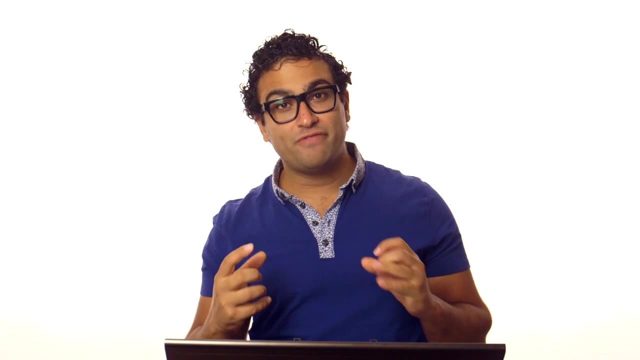 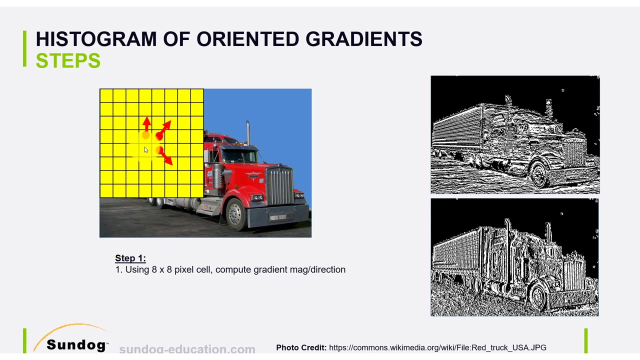 Again, square root, gx squared plus gy squared and tan minus 1, gy divided by gx will give me the angle and will give me the magnitude value as well. So I have the magnitude and I have the direction. All right, great. So now pretty much I have. for each pixel I have a value which. 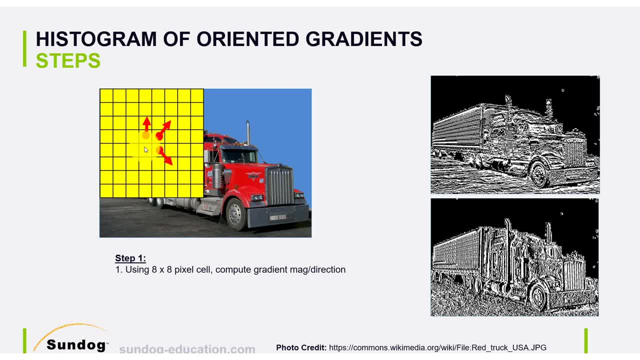 indicating the length of that line, and I have an angle or orientation, okay. So the beauty about the histogram of oriented gradient is that I can take the oriented gradients that I have and can kind of draw a histogram of it, the distribution of it, in a way, okay, Which is 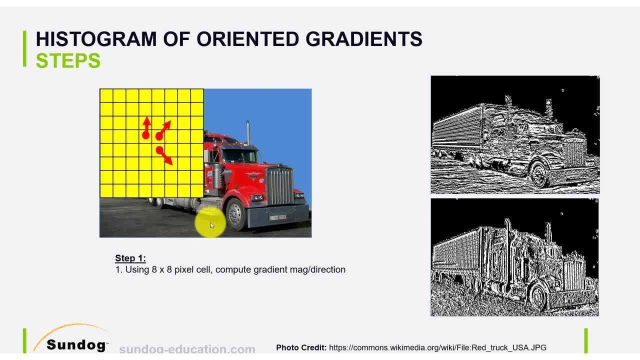 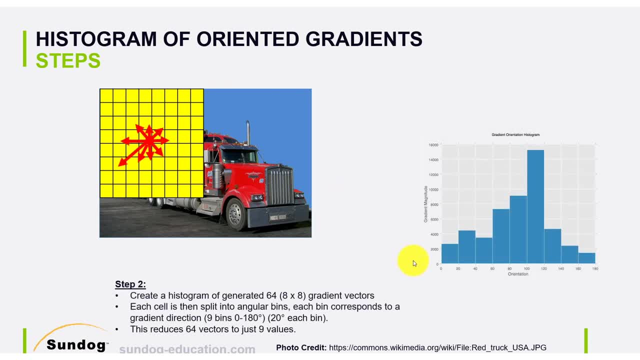 simply put how many, for example, gradients within that cell that has 45 degree angle And that's where I'm going to draw my histogram of oriented gradient per se, And that's the beauty of it. So that's kind of the orientations, which is you know, I'm going to divide simply. 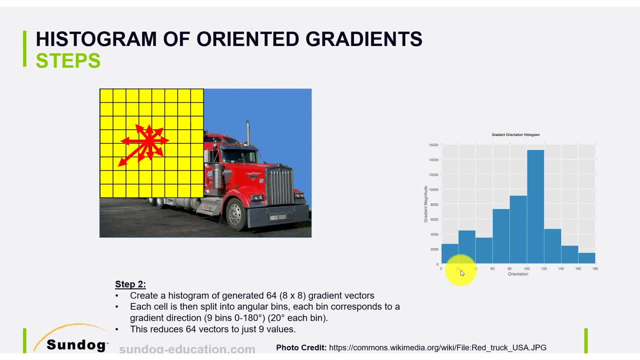 the 180 degrees to, let's say, from 0 to 20,, from 20 to 40,, and so on, so forth, And that's the beauty of it. So that's kind of the orientations, which is you know. 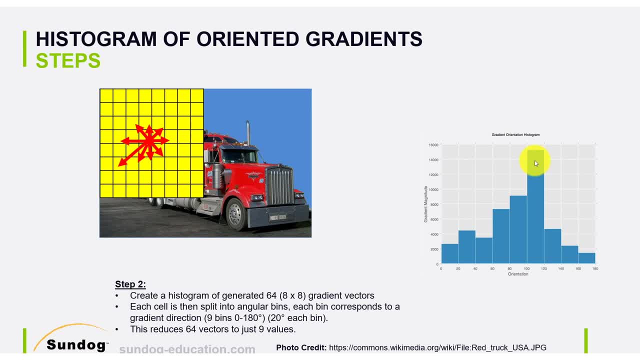 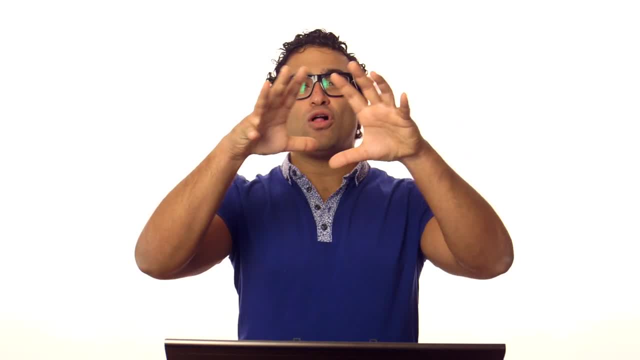 and here I'm going to plot all the gradient values or gradient orientation magnitudes. Here I'm showing magnitudes, here I'm showing values, And that's the amazing part of it. Now I can put all the information within that pixels, within, let's say, the 8 by 8, which is 64,, I can simply 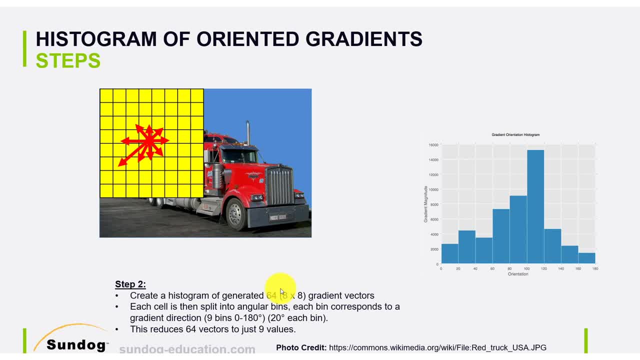 kind of combine them or like zip them in a way, you know, like kind of. again, as you obtain a zip file, okay, Compress them in a way to obtain these kind of values, which is again what we call histogram of oriented gradient. Okay, in another fashion, I can even view all. 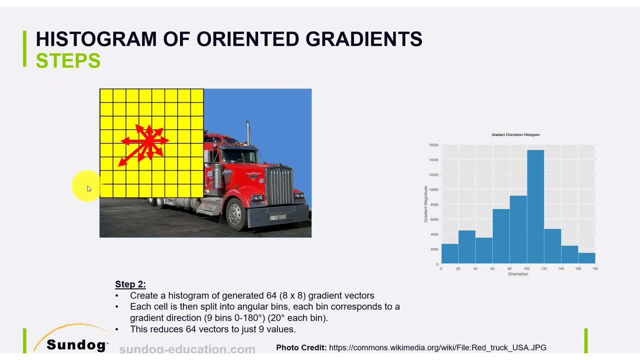 these pixels within all that range, within all these cells, but kind of, you know this format, which is okay showing okay. at different angles I have different magnitudes. That's the magnitude for, let's say, a specific angle. This is a magnitude at 0 angle. This is a magnitude at 90. 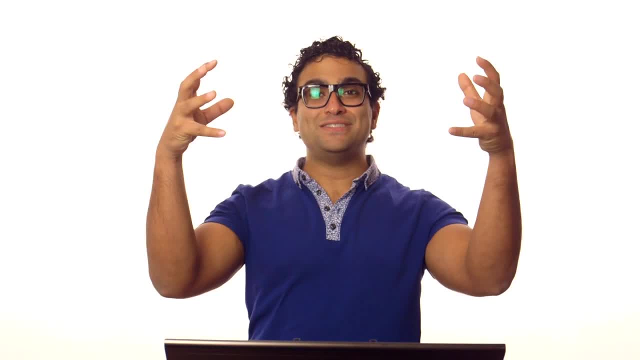 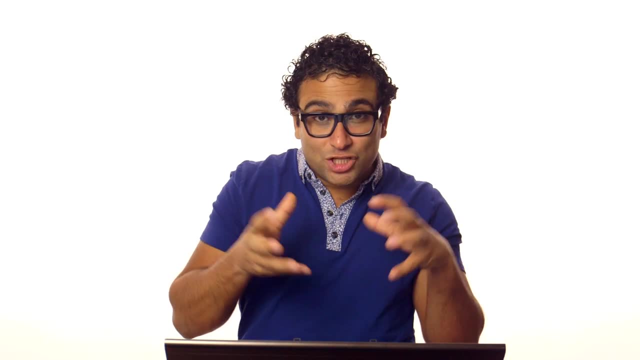 angle degrees and so on, so forth, And that's the beauty of it. Now you condense all the image in kind of these, like you know, like a, like a like image, in a way, in a very kind of, you know, compressed form that you simply reduce 64 vectors. 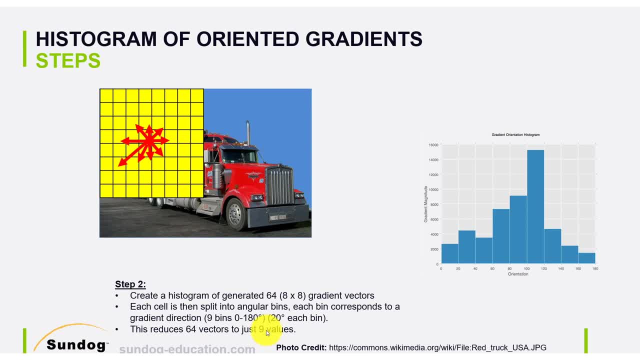 in kind of just nine values, which is the beauty of the what we call histogram of oriented gradients. All right, Okay, Sounds great, So let's take again more, a little bit more, look. I know it's a little bit, sometimes a little bit confusing, So let's take a look at what can. 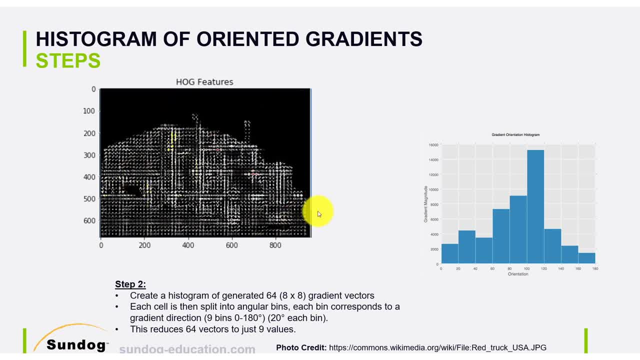 what does a Hawk feature look like? Actually, that's what a Hawk feature is going to look like. That's a truck, That's how, basically, computers, or you know, machine learning algorithm, computer machine, we're going to, we're going to know a truck. Okay, So we humans, we can. 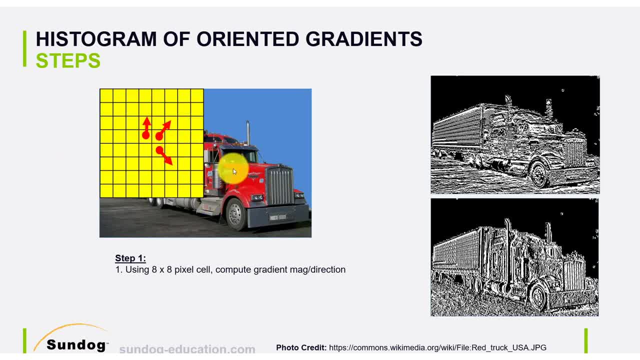 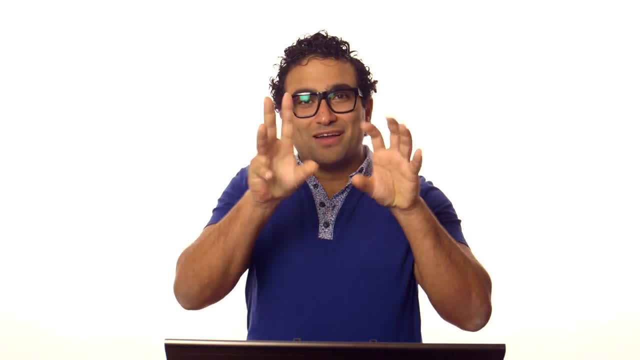 okay, detect. okay, this is a truck. Okay, Using just, you know different colors, different features, And that's the Hawk features, That's how you can compress all the information using these kind of you know, like like stars, you know white stars in a way, And that's the Hawk. 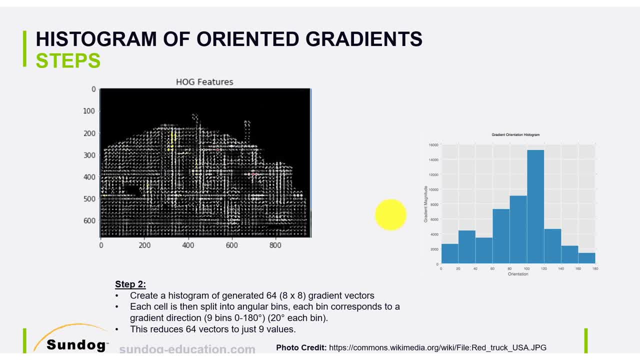 features. And that's how can you choose or take all this, basically information, feed it in a classifier to detect if you see a truck or no. Okay, All right, That's great Again. I know it's a little bit confusing. Let's see what. what can we expect Again? 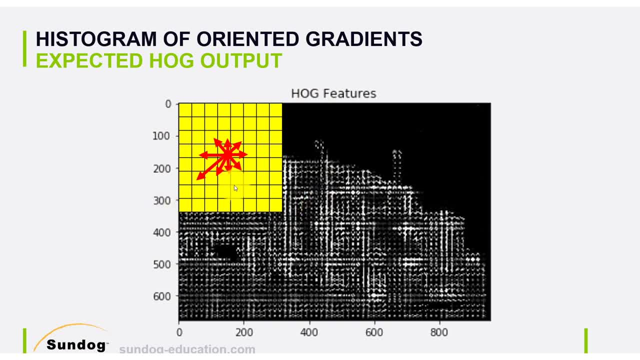 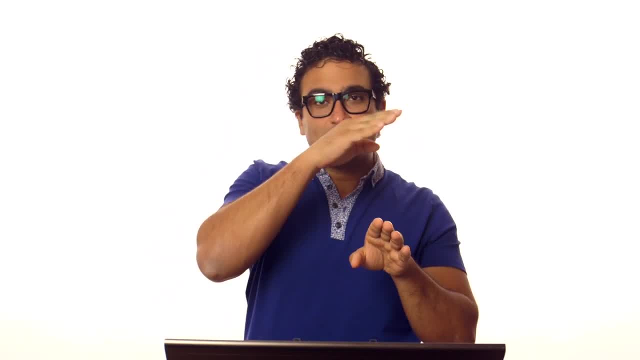 so we're going to take again a window, kind of a, like a. we'll call it cell And each of the cells we're going to come up with this kind of star value indicating different gradients, magnitudes and different angles. We're going to again shift again. We're going to get another.